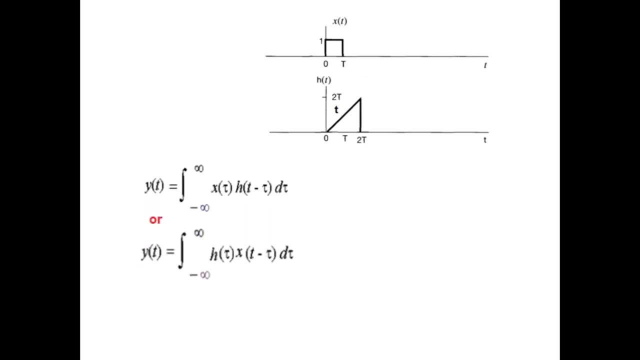 We, and these are the two formulas that we have. we discussed this formula, And there is another way of writing this, that is, in this case we shift X function, not H function. So that is what we'll do here, because H function. 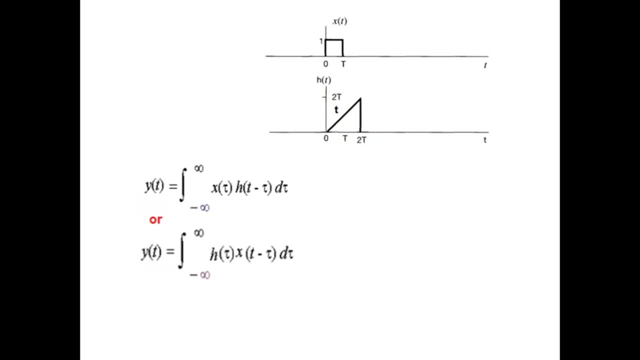 is difficult in this case. So we'll shift the X function. So our arrangement will now be like this: This is Ht and here is Xt. We'll flip this and shift this function. So we'll do this, Case number one, or step number one, change the variable from t to tau, So everything. 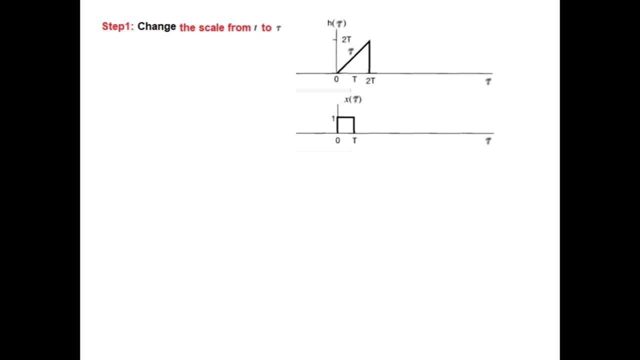 has now been changed from t to tau. Flip one of the signal, that is, the, we'll now flip Xt signal around X axis. So from here we flip it like this, So this becomes the flipped signal, And since it is in the negative direction, so it will be X minus tau, And now we'll play. 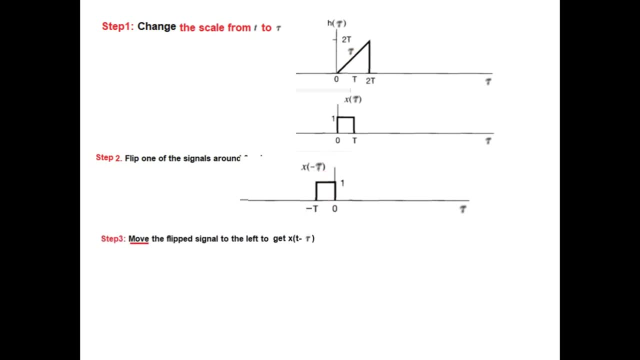 with these two signals: Move the flipped signal to the left to get Xt minus tau. Actually we are adding t here and t here, So it'll be t and t minus capital T. So we moved it to the left: T and T minus capital T. And as we did in the first case, first example: if you assume 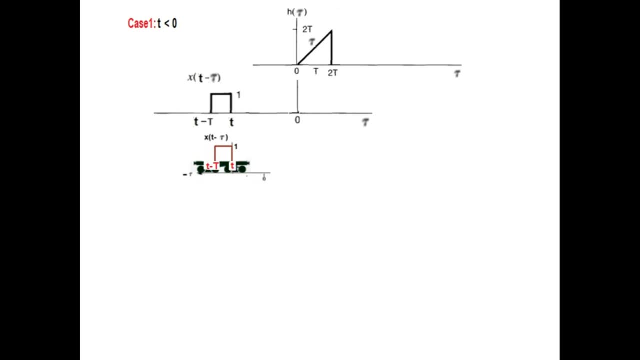 it to be mounted on a trolley. it will be much easier for you to comprehend. So this is T, and this is T minus capital, T. And now we'll pull the trolley gradually till such time it starts overlapping. Okay, Now for T less than zero. so this T or this T less. 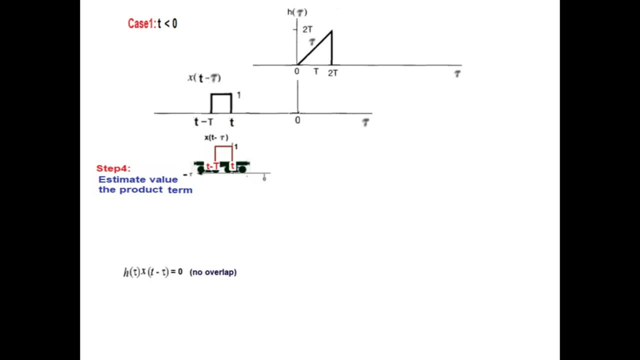 than zero. there is no overlap. So the product will be zero, no overlap, And hence the estimated range. we can say it is minus infinity to T or zero, I'm not very sure What range you will call it Then. it's minus infinity to zero, And then the output from: 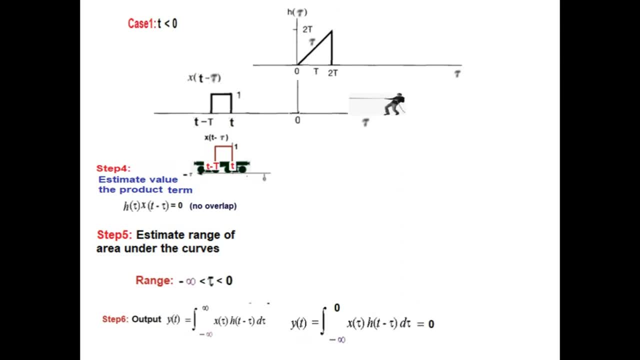 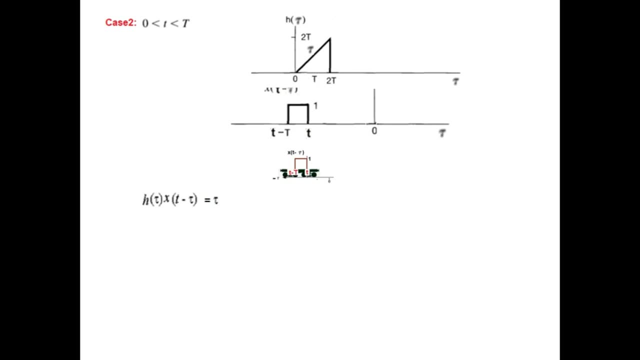 the equation output will be zero. Okay, Now case two. we have pulled it slightly. Now T is between Zero and capital T. So case number two: T is between zero and capital T. You have to look at this T, the trolley T. It is between zero and capital T. So that is our first case. 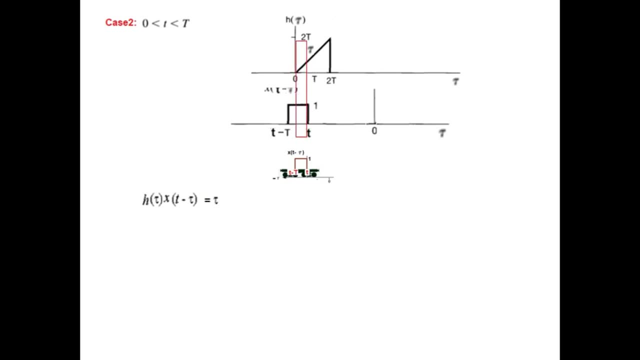 And we have some overlap. Here is the overlap. You can see, this is the overlap. So our multiplication will be This function, which is T all the way. So T multiply by one, So this is equal to T. T multiply by one is T, So this is the product. And now we estimate the range of the area under 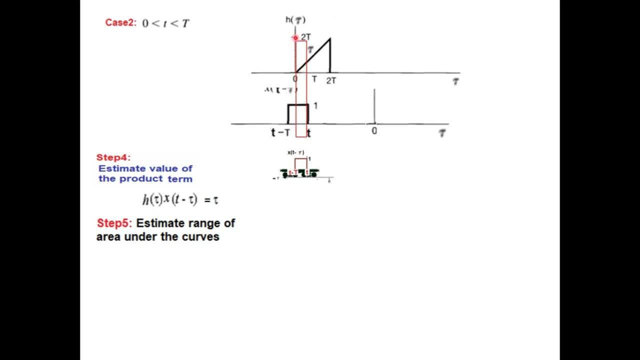 the curve. So now this is the area under the curve. This is showing The overlap, What is defined clearly? Zero is defined clearly. So one of the starting point will be zero. End point is not defined here clearly, but it is defined here clearly. 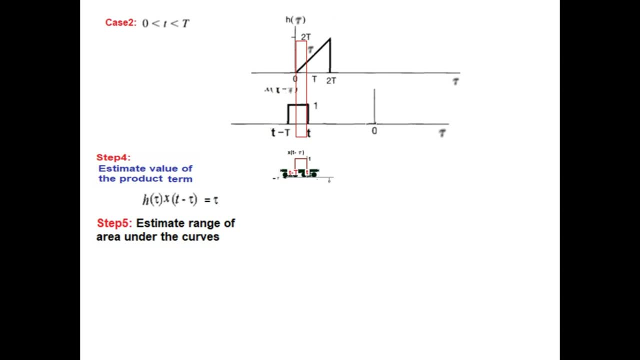 It is small t, So our range of tau will be from zero to T. So tau is from zero to T. That is will be the limit limit of the integration for the output. So output formula, Put the limit of integration, Put the value of the multiplication which was tau Integrate, So it will become tau. 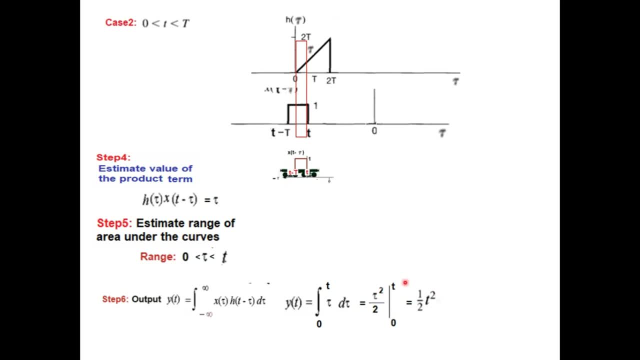 square over. 2. Put the two limits, So the final answer is half t square. So this is case number 1.. Now let's pull it further. So now we have pulled it So that t comes between capital T and capital 2 t. So this is our case number 3.. The t is between capital. 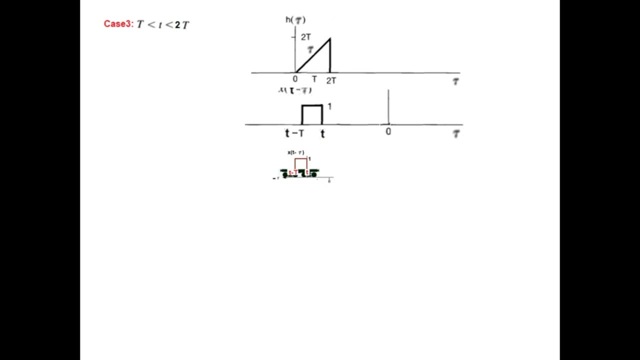 t and capital 2 t. The overlap, Complete overlap Of the bottom signal. The slope is still tau And this has an amplitude 1.. So the multiplication will be tau times 1, which is tau. So the multiplication of the product gives tau. Now, 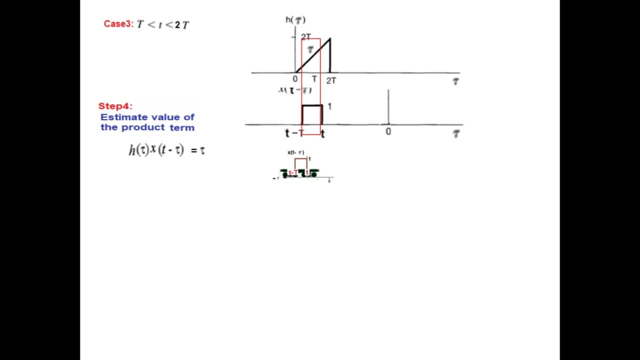 the range of integration. Now you can see it is not clear here what is the value, which is not clear here what is the value. But it is clear here that it is t minus capital t, And here it is t. So these two will now be our range of integration. So the range for 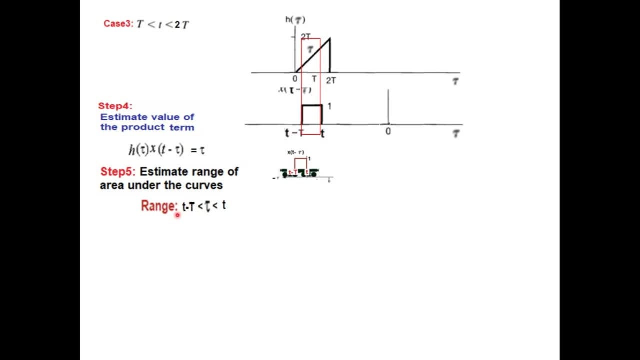 tau is t minus capital t And the other end it will be t. Okay, So integrate. these two are the limits And tau is the value. So will integrate tau square over 2. These two limits And putting the limit, And solving, And solving, And solving You get the final value. So this: 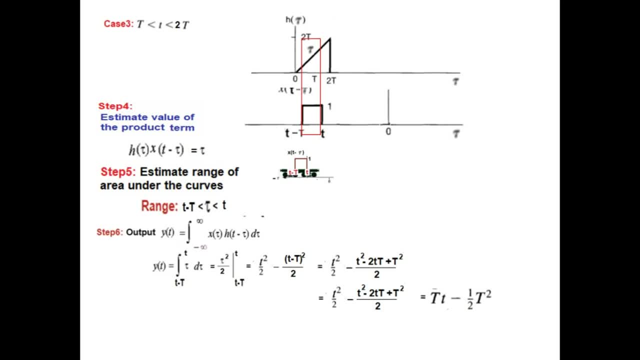 is the final value For case number 3.. pull it further. okay, now we have pulled it beyond 2 capital T and in between 2 capital T and 3 capital T. so this is here. so the range is now from 2 capital T to 3 capital T, and this is the overlap. the multiplication remains same. 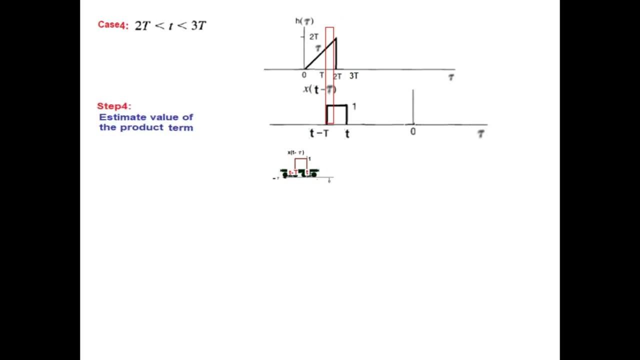 tau multiply by 1, so multiplication is tau. and now the range of the limit. so let's see this point is not defined, so this will take as here it is defined clearly. so it is T minus capital T, but this point is not defined. here it is. 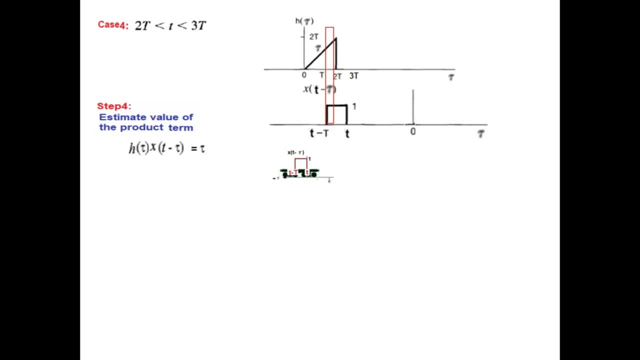 defined clearly here. so it is 2 capital T. so our two limits of tau will be T minus capital T to 2 capital T. so this is the limit of the range. and now I put in the equation these two limits. keep in mind this one and this one, integrate and solve. so the final answer. 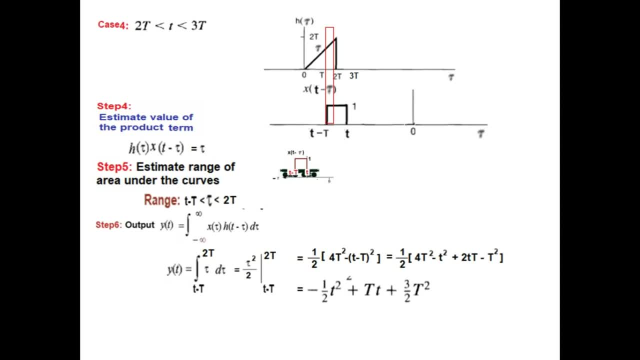 gives us this: that if you add a value of 2 capital T, then we have impossible decision. in my simple equation, you shall not get a square root of 2. that's why перв term isなんか n taki of μας stamat. he will give n, as as shown here. 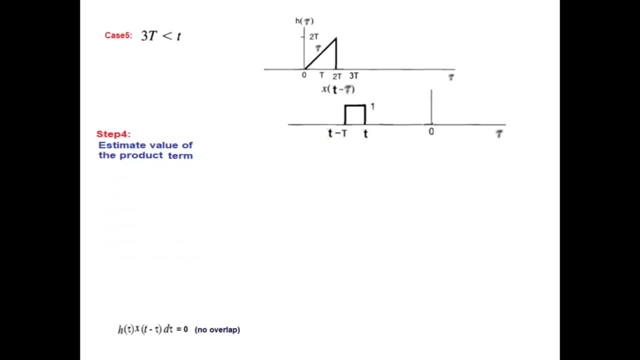 one more pull the moment he goes beyond 3 T. there is no overlap, so output will be zero. this has Educated from 3t, hopeted that it becomes equal when sending this over. if given X is n minus 2, N, that can be God. what if we have n? will omitted instead and we just 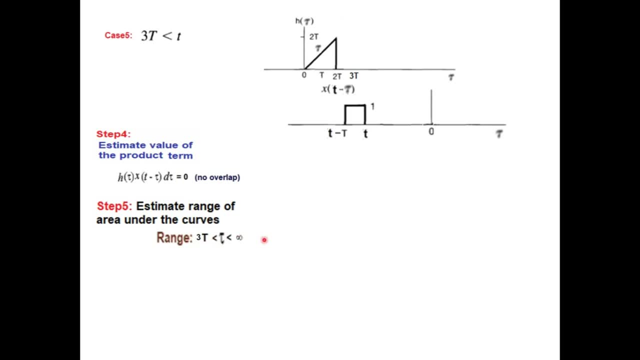 if you have n, it becomes n as any possible. this one c 죄 descibe, you can just say so now- of that�� phone to a periodках, so you'll never have a tested this time. media does not matter to infinity, or we should write. 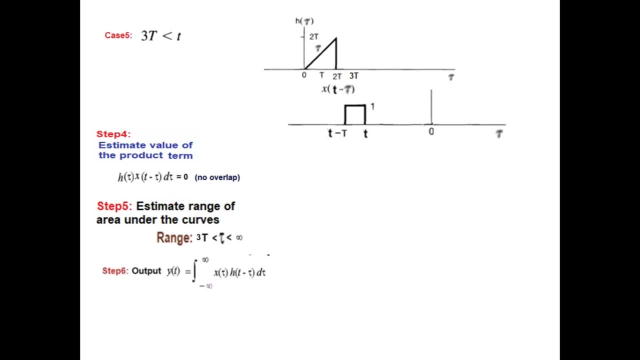 just no range. but anyway, since multiplication is zero, therefore the output.